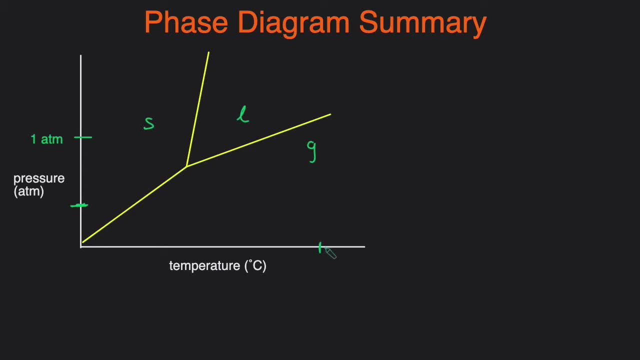 gas at that pressure and that temperature. Some other points that you you need to know. we have the triple point right here, which is the intersection of the three lines, and the triple point that's that's the point in which all three phases exist at equilibrium. That means that at this particular 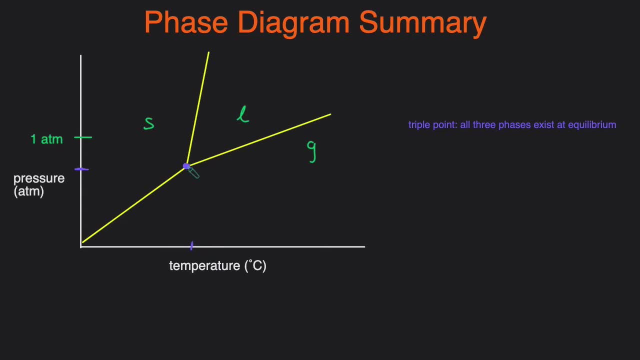 pressure and that particular temperature. all solid, all three phases- solid, liquid and gas- will exist. Another point that's useful to know is this point right here and that blue point. this is called the critical point. The critical point can be broken down into the critical. if you trace it down here, this would be. 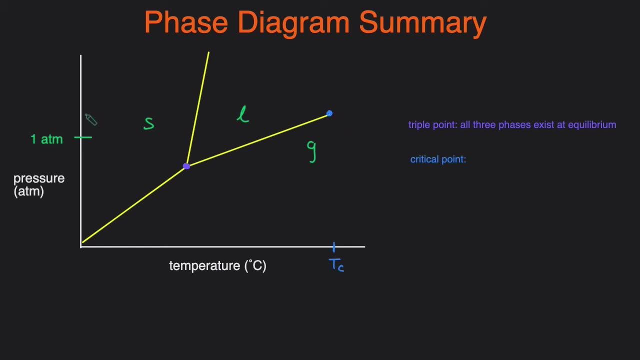 the critical temperature, and if you trace it over here, that would be the critical pressure, And then if you bring the points up and then bring the line over, then you get this region right here. So what's so special about the critical point is that just in this region, above the critical point, you no longer can differentiate. so you, you no longer. 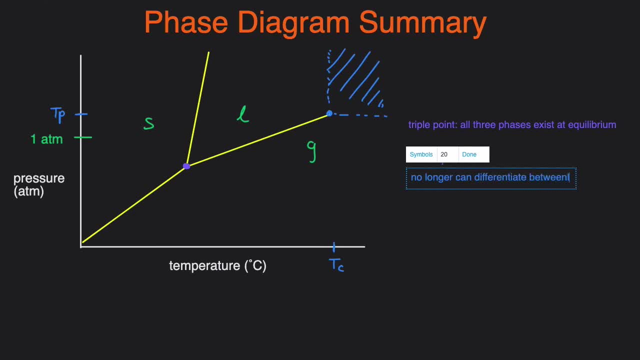 can differentiate between the liquid phase and the gas phase and instead they sort of combine to become a super, a new phase called supercritical fluid. So that's another point that's important to know. And then, lastly, you need to know all the phase changes, that that can occur. 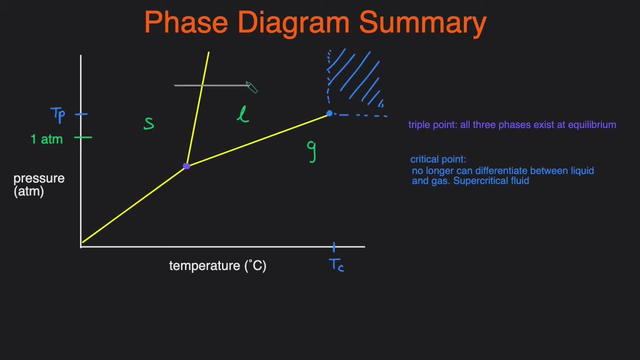 If you're going from a solid to a liquid, that's just called melting, And then if you're going from the liquid to the solid, that is called freezing. If you're going from the liquid phase to the gas phase, that's called boiling, or also called 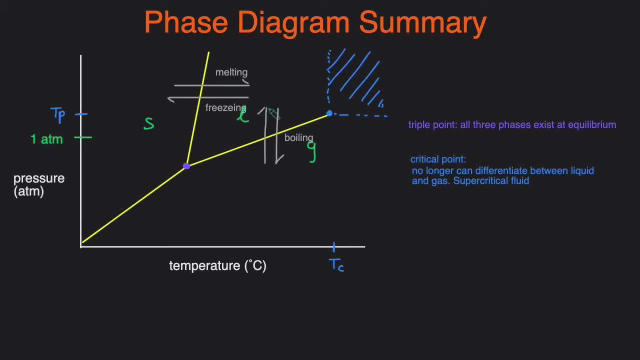 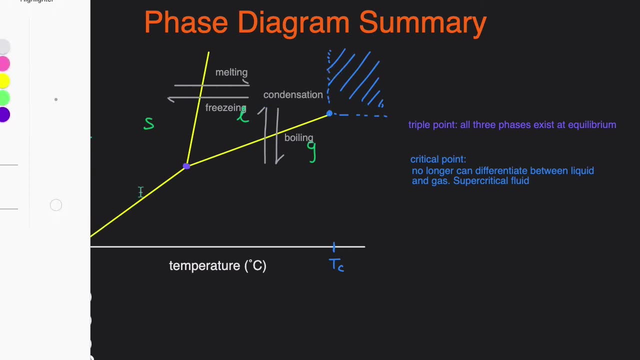 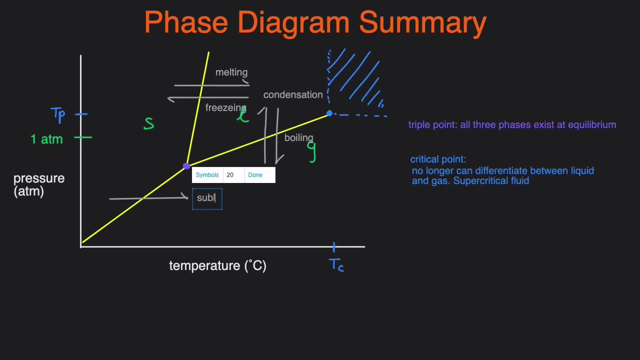 vaporization, And then if you're going from the gas phase to the liquid phase, that is called condensation, And then, if you're going from a solid to a gas, that is called sublimation. And lastly, if you're going from a gas to a solid, that is called deposition. 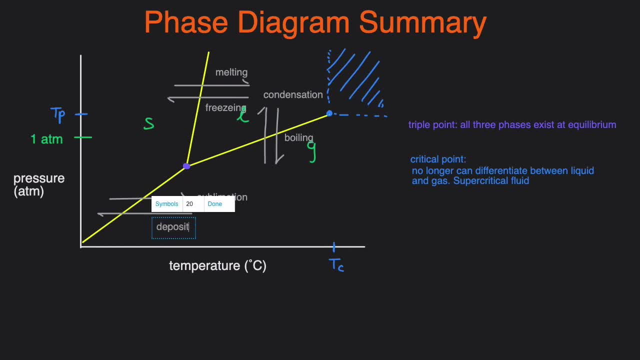 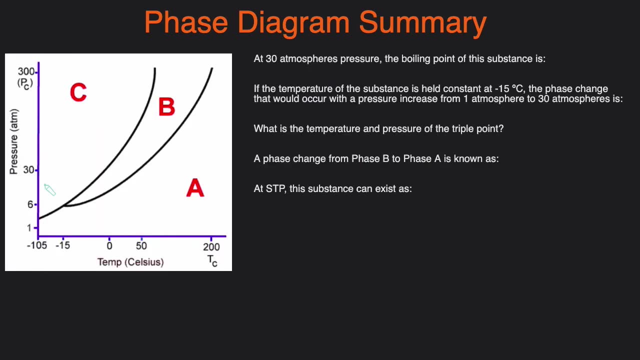 Now let's take a look at some practice problems to apply what we've learned Here. we have a phase diagram with a, b and c. The states aren't labeled, so let's first take a look at the phase diagram. So let's first take a look at the phase diagram. 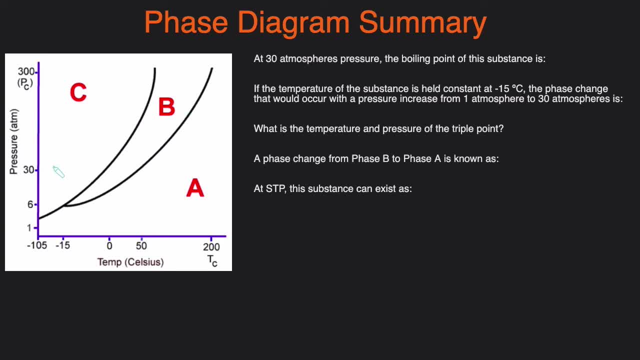 Here we have a phase diagram with a, b and c. The states aren't labeled, so let's first label states. We know that to label states we go from left to right and that'll be solid liquid and gas. So c is a solid, b is a liquid and then a is a gas. 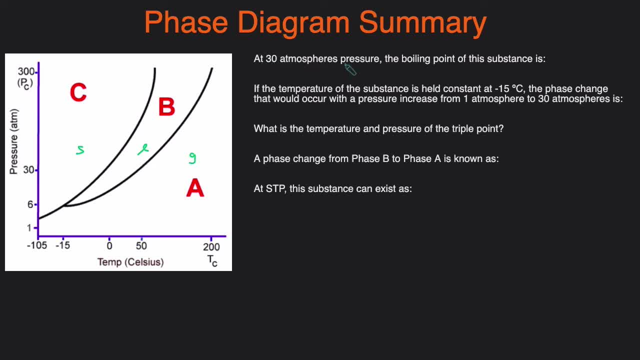 So the first question it asks: at 30 atm the boiling point of the substance is. So we're at 30 atm and boiling occurs when a liquid becomes a gas. So we just trace that over and then and then trace that down, So that'll be 50 degrees celsius And that'll be the boiling point. 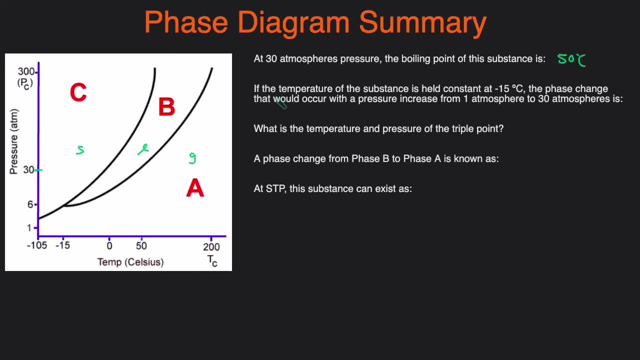 at 30 degrees atm. The second question asks: if the temperature of the substance is held constant, negative 15 degrees celsius, the phase change that would occur when the pressure goes from one atm to 30 atm is. So we're given a temperature negative 15 degrees celsius And it asks: what's the phase? 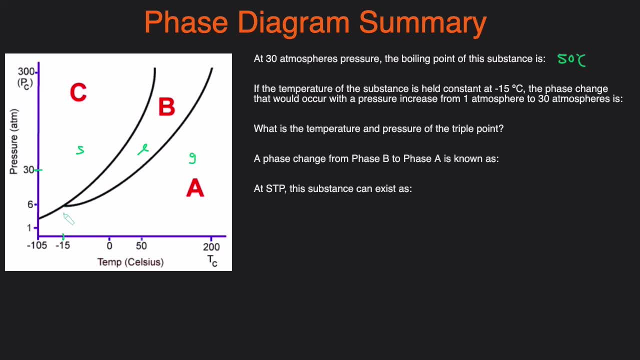 change that will occur when it goes from one atm to 30 atm. So we're starting at one atm, We're going to 30 atm, So you're going upwards And you can see that's going from the liquid. a is a liquid. 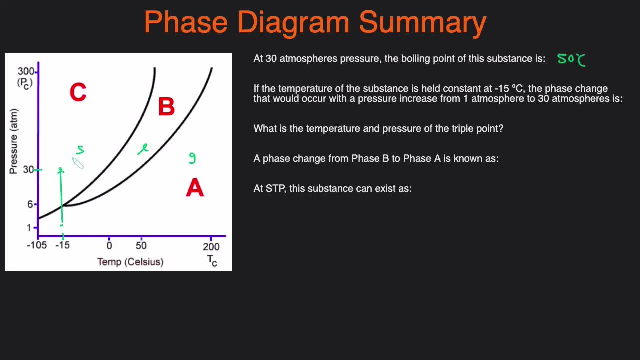 C is a gas, so it's going from- sorry, it's going from a gas to a solid. A is a gas and C is a solid, So gas is solid. that would be deposition. Then the next question asks: what is the temperature and pressure of the triple point? 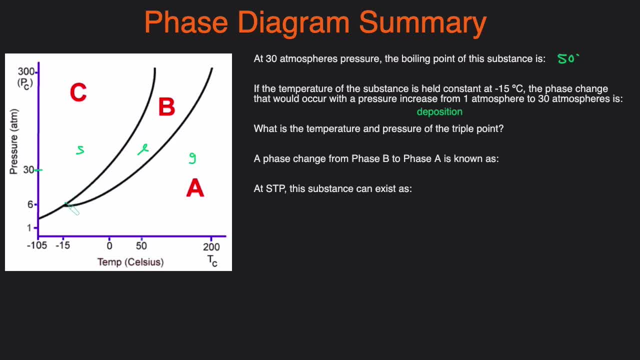 So we know that the triple point is the point where all three lines intersect, and that's going to be this point. And so then the pressure would be 6 atm and then the temperature would be negative 15 degrees Celsius. So 6 to atm and negative 15 degrees Celsius. 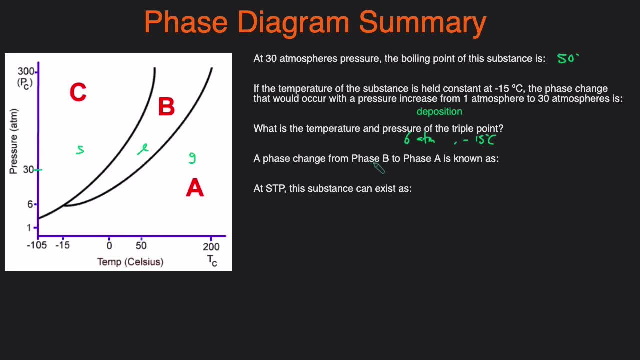 Next question: a phase change that occurs from B to A is known as: so now we're going from B to A, and B to A is just a liquid going to a gas, so that's just known as boiling, or we can say vaporization. 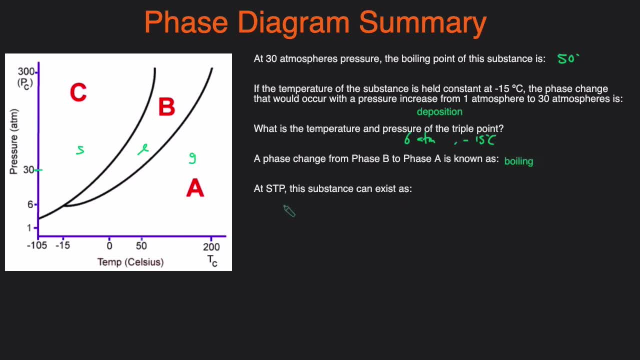 And then, lastly, at STP, the substance can exist as so. STP is 0 degrees Celsius and 1 atm. So let's trace that 1 atm, 0 degrees Celsius. that's at this point, and that's A, and A is a gas.